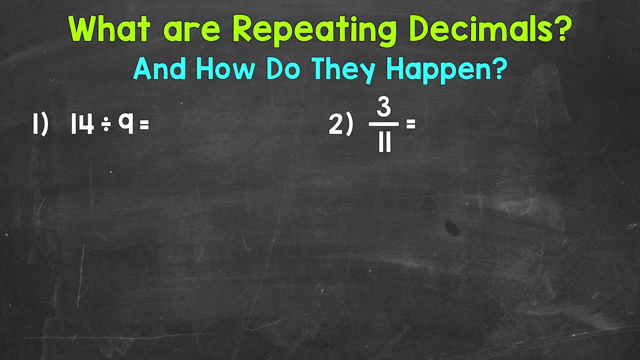 So let's set this problem up: 14 divided by 9.. And we'll go through our process. So, 14 divided by 9, how many whole groups of 9? Out of 14,? well, 1.. 1 times 9 is 9.. 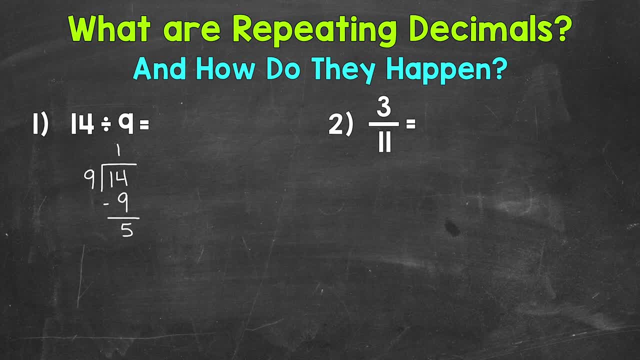 Subtract, we get 5.. Now we want to keep this in decimal form, so we need to continue on with our division process. The goal is to get a clean cut zero here, and that's when our decimal or answer will terminate. 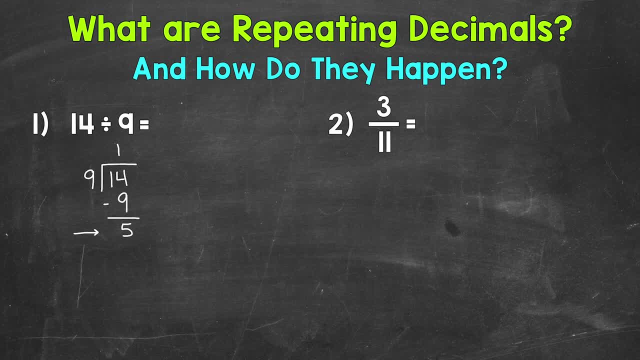 But in the case of this problem it's going to be a repeating decimal, So let's look for a pattern here. Now, since we want this in decimal form, we need to place our decimal after the whole number- so after the 14, and bring it straight up into our answer. 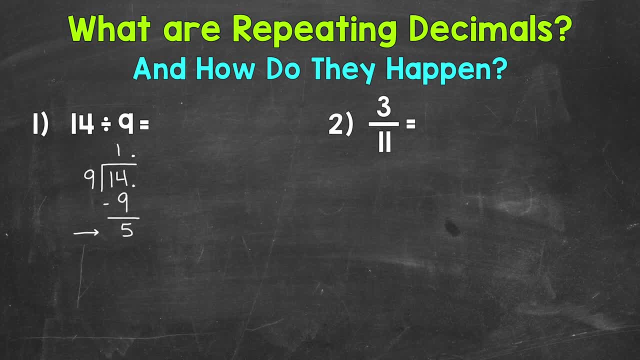 Once we do that, we can extend with placeholder zeros here. These do not change the value of the problem. This is equivalent to 14. still Now we can bring that zero down and we have 50 divided by 9.. So how many whole groups of 9 out of 50?? 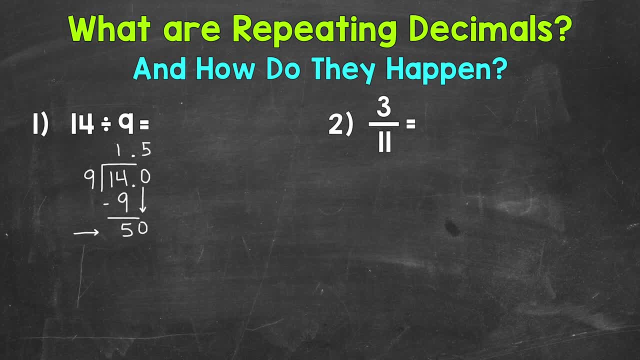 Well, 5. That gets us to 45. Multiply 5 times 9, 45. Subtract, we get 5.. So we need to continue on. So we can use another zero. Bring that down And we have 50 divided by 9 again. 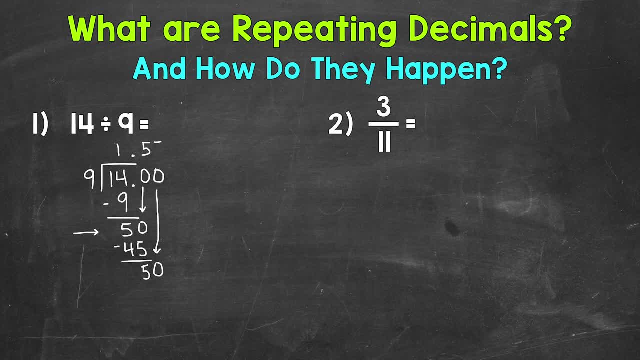 So how many whole groups of 9 out of 50?? Well, 5.. 5 times 9 is 45. Subtract: we get 5. And you're probably seeing a pattern. so we can use another zero Subtract: we get 5.. 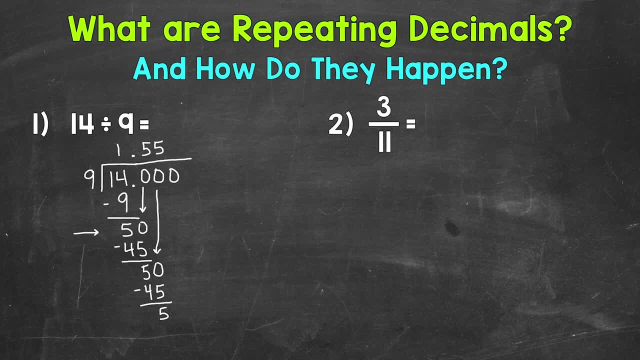 And you're probably seeing a pattern, so we can use another zero. Let me extend this bar here. Bring that zero down And we have 50 divided by 9 again, which is 5.. 5 times 9, 45.. 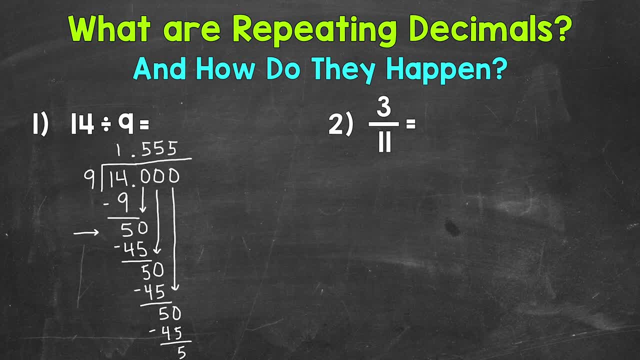 Subtract, we get 5.. We can use another zero, And that pattern is going to continue on forever. So we get 1, and then repeating 5s that go on forever. Subtract, we get 5. And that pattern will just continue. 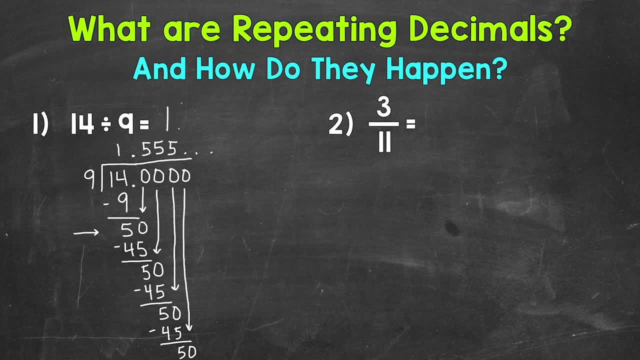 So we can express our answer as 1, and then 5 repeating. So what we can do, we can put this in bar notation is what it's called. We put a bar above that 5, and that shows that the 5 repeats. 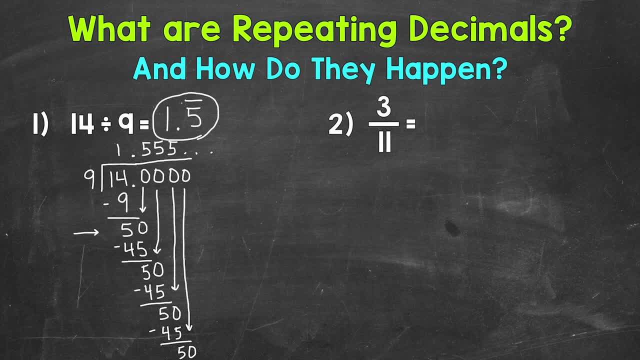 So our answer: 1 and 5, repeating. Let's do another example and move on to number 2, where we have 3 elevenths. So we're going to take that fraction and convert it to a decimal. We do that by using division. 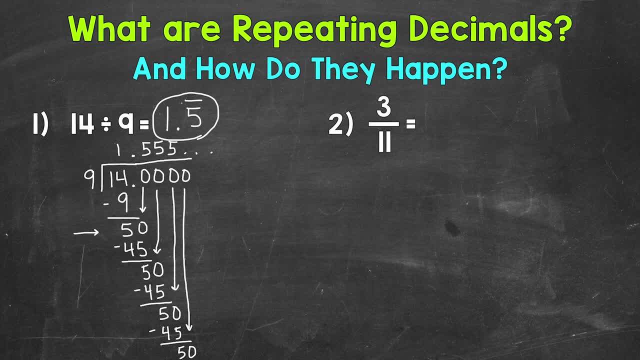 So we do 3 divided by 11. Let's write that out and go through the process. So 3 divided by 11. And we start our process by seeing how many whole groups of 11 we can pull out of 3.. 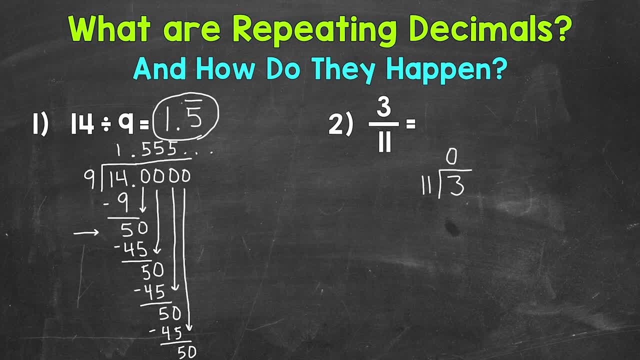 Well, we can't do that, so let's put a zero there. Now, in order to continue on and put this in decimal order, we're going to have to do this again: Subtract, we get 5. And put this in decimal form. 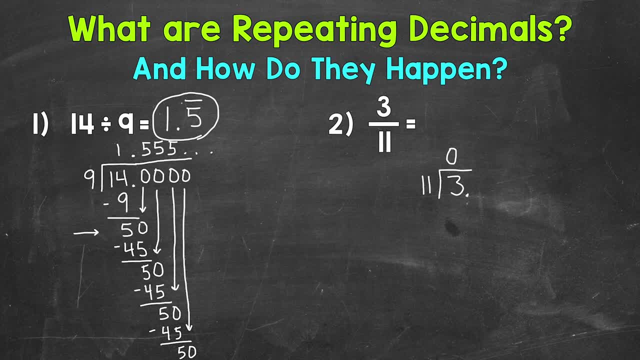 We need to place our decimal after the whole number and bring it straight up into our answer. Now we can use a placeholder zero to keep going And we have 30 divided by 11.. So how many whole groups of 11 out of 30?? 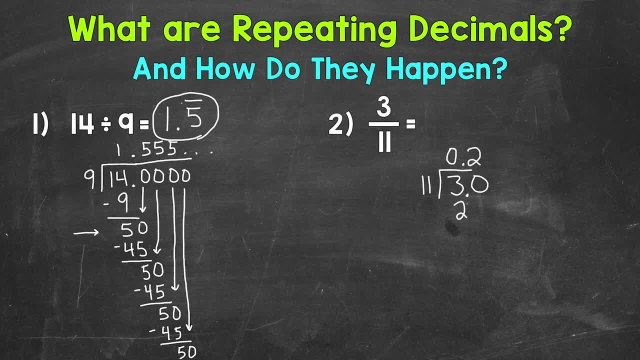 Well, 2.. 2 times 11, 22.. Subtract, we get 8.. Remember, we want to look for a clean-cut zero. That's when we know that the decimal is in decimal form. The decimal is going to terminate or end. 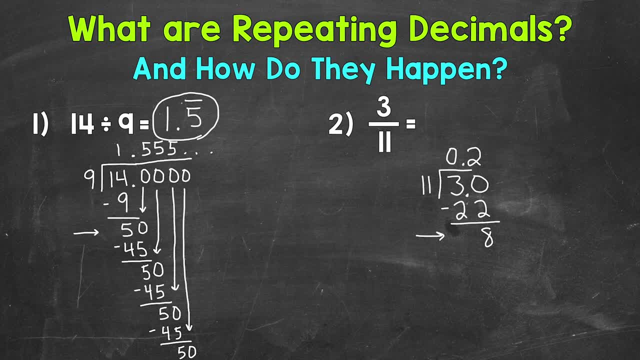 We have an 8 here, so we need to continue on. Let's put another zero that we can bring down. So now we have 80 divided by 11.. So how many whole groups of 11 out of 80?? Well, 7.. 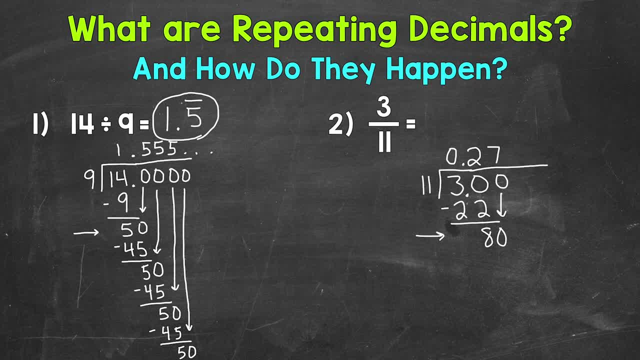 That gets us to 77. Let me extend this here. 7 times 11 is 77.. Subtract, we get 3.. Let's use another zero. Bring that down, So we have 30 divided by 11.. How many whole groups of 11 out of 30?? 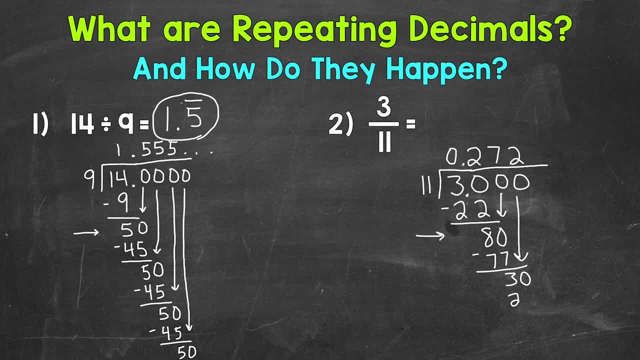 Well, 2.. 2 times 11 is 22.. Subtract, we get 8. And you may start to notice a pattern here as we extend with another zero. So 80 divided by 11. Well, that's 7.. 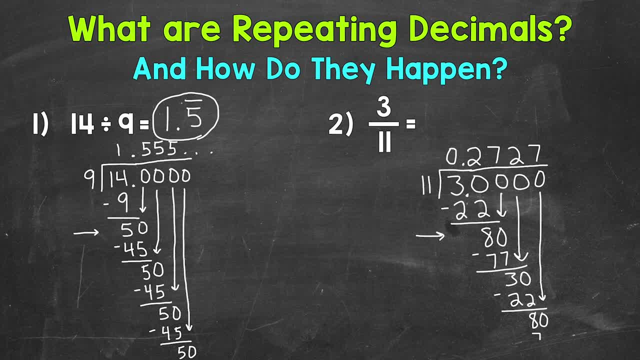 That gets us to 77.. 7 times 11,, 77.. Subtract, we get 3 again. We can extend with another zero And that pattern is going to continue on forever. So we get 0.27 repeating here. 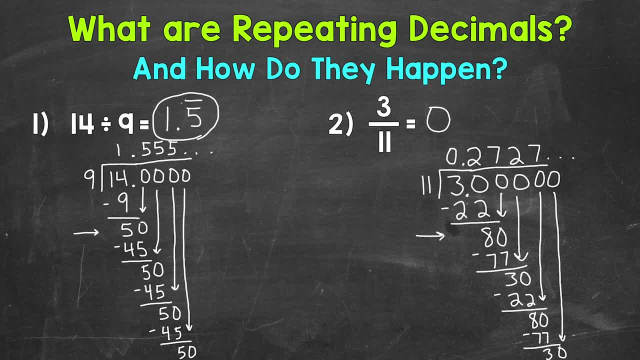 And we can express this by writing 0 decimal And then the digits that repeat. Well, we have 2, 7, 2, 7, 2, 7.. So the 2 and 7 repeat. So we put a bar above the 2 and the 7.. 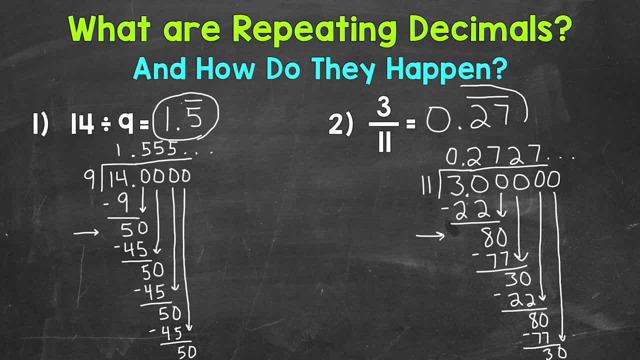 If we have a group of digits that are repeating, you put the bar above that group that repeats, So 0.27 repeating. So you can see that as we go through our long division process we have a pattern that continues on forever. 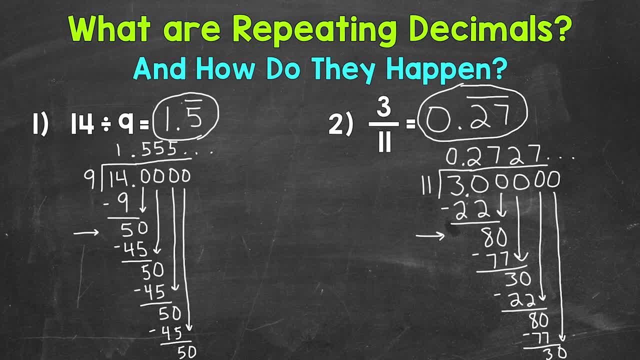 And that gives us our repeating decimals. So hopefully that gives you a better understanding of repeating decimals and how we get repeating decimals. So I hope that helped. Thanks so much for watching. Until next time, peace.